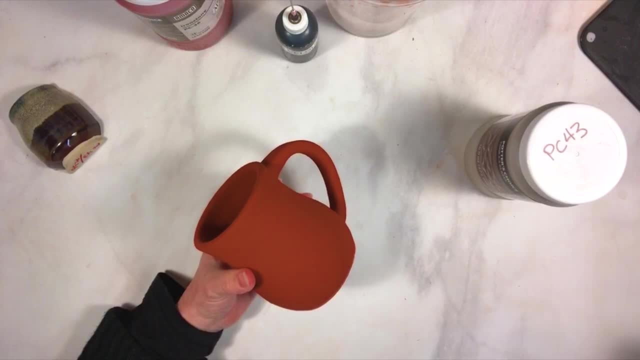 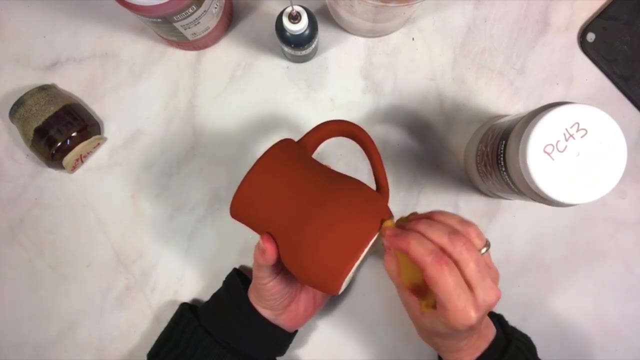 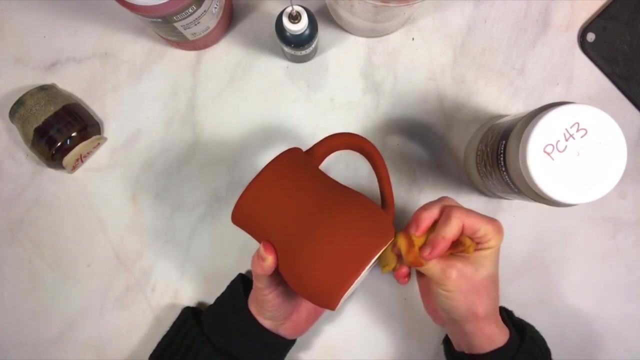 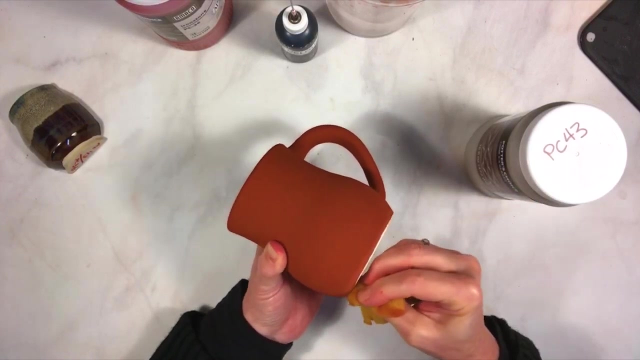 bit of sponge stuck to my mug. If you're rejoining me after seeing the first video, part one, live, you may have noticed that the video cut out kind of abruptly and there wasn't really anything important that was missed, Just finishing up the glazing and saying come on back for part two. So I'm going to clean. 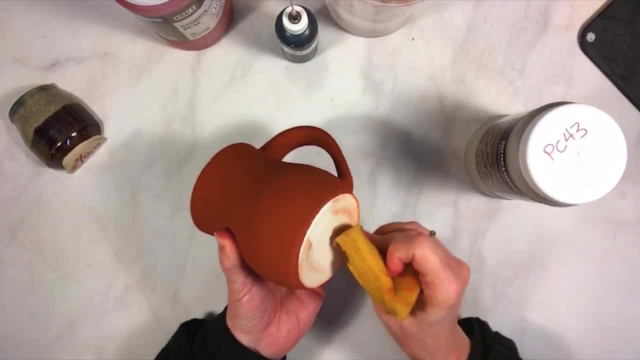 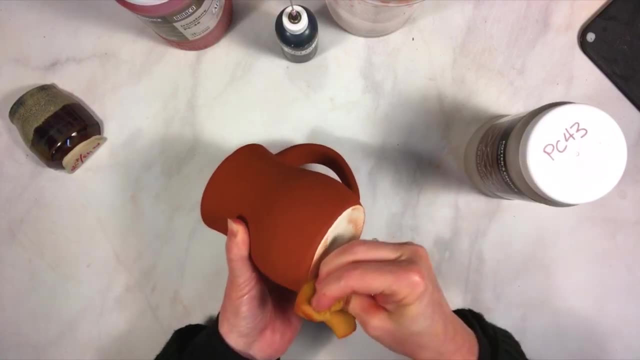 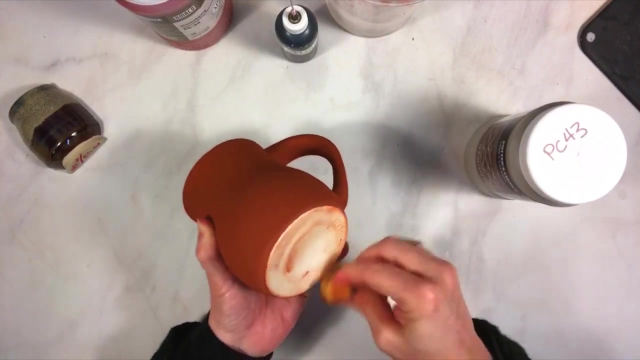 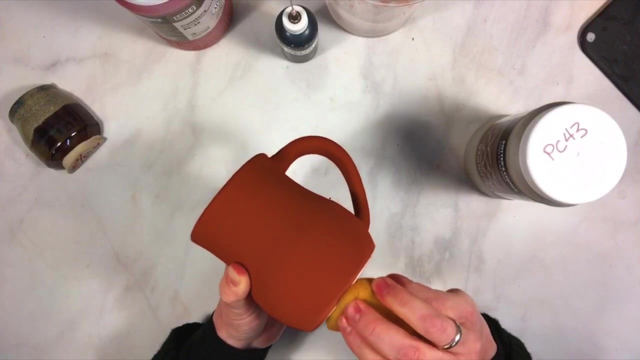 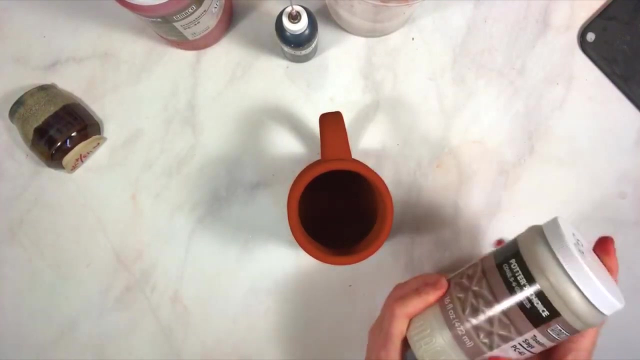 up the bottom with the Toasted, with the Ironstone, Make sure that it's all off the all off the foot. Being an iron rich glaze, it does tend to smear and stain the foot, which can be a pain in the butt, But it's okay. So here we go, Cleaned. I've got my PC-43 Toasted. 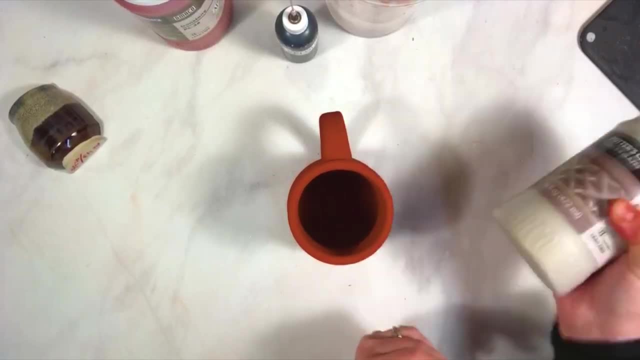 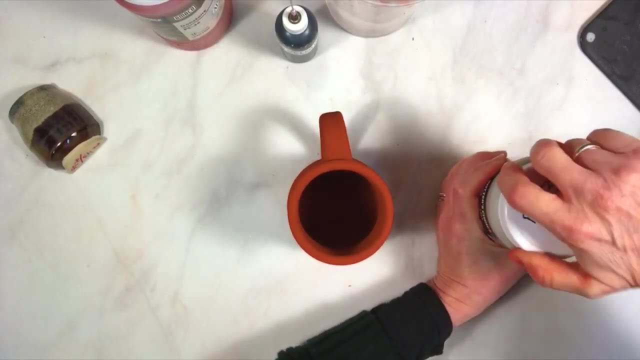 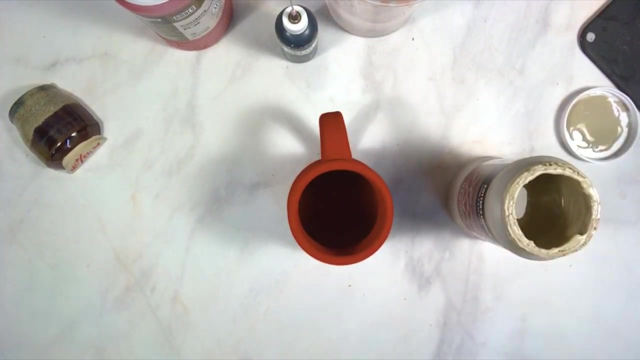 Sage Shake, shake, shake, Probably shaking the table as I do this. So I think I know why the video cut out at the end last time. I think that we will have better results today- well this afternoon- than we did this morning, So I'm gonna go with the same size of brush, You can see. 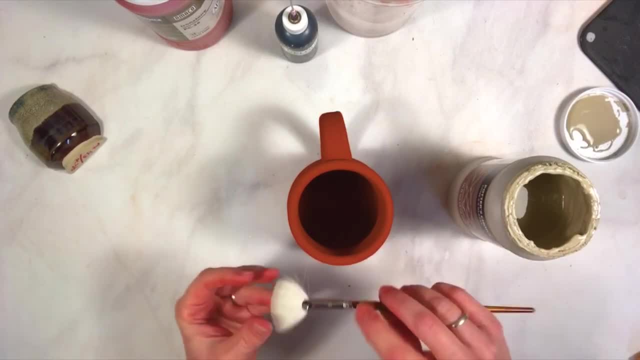 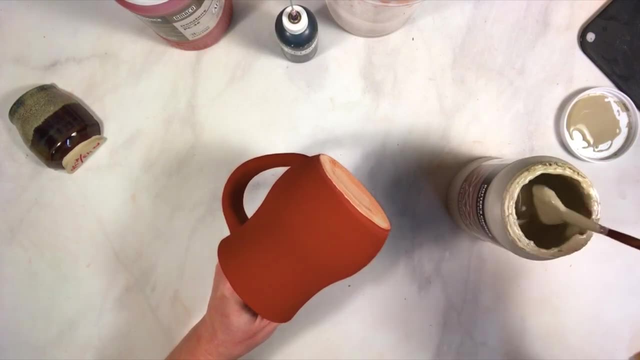 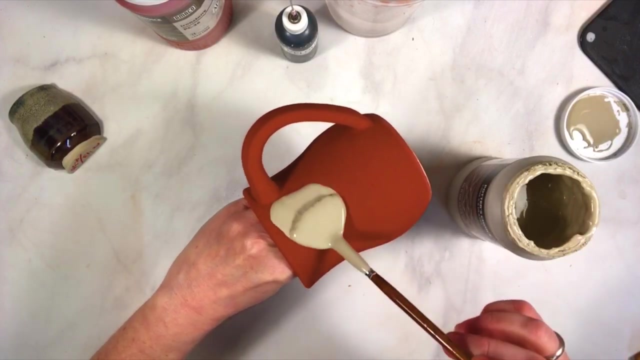 This is a new, very, very new brush. The bristles haven't been stained with iron, like all of the rest of my brushes tend to do, And for this I'm going to do kind of a swoop with the top coat of glaze. 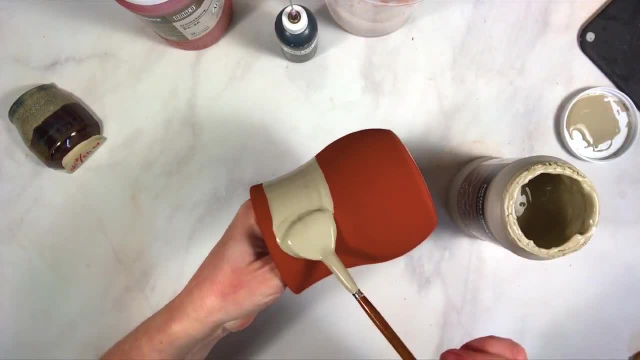 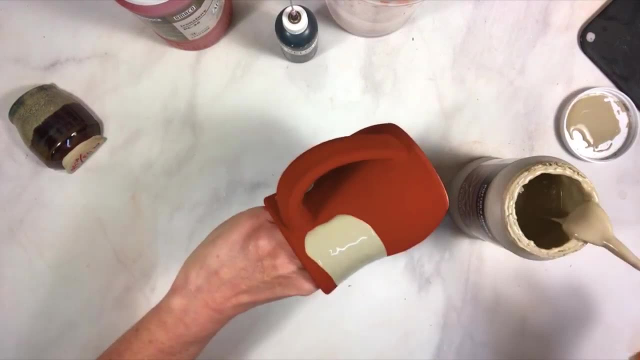 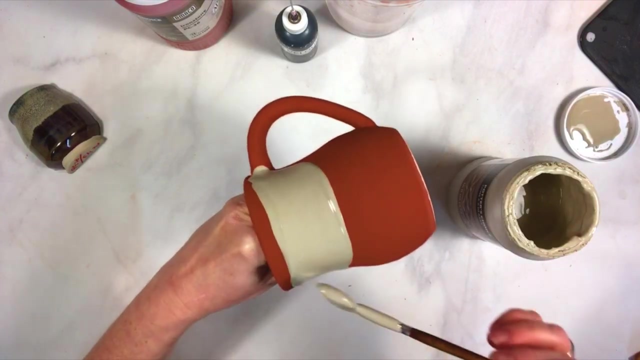 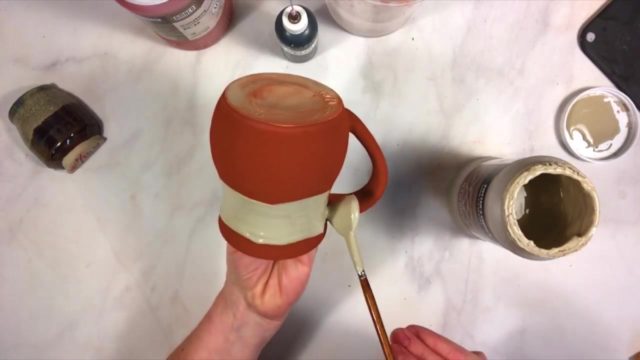 I'm going to give it a little bit of space at the top. As I've said before, the question with food safety is that we don't test combined glaze combos. We just can't because of the number of variables. Do a little bit down the handle. 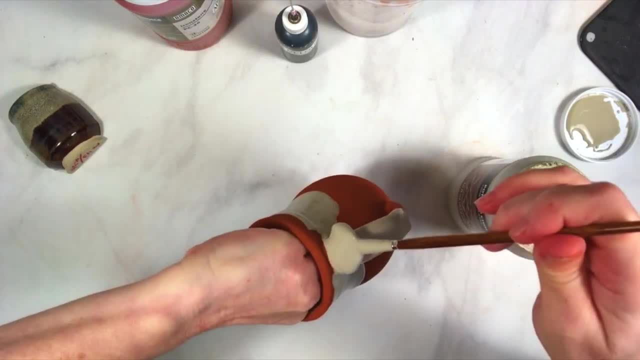 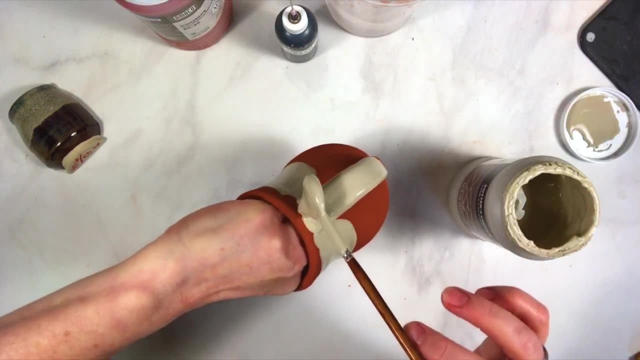 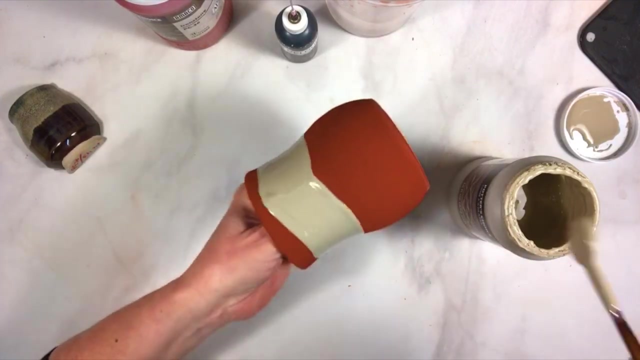 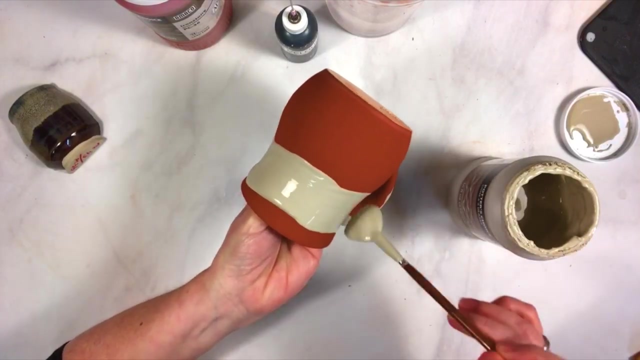 So if you're wanting to be assured that the glaze passes our food safety testing, as prescribed by the FDA, we suggest you use a single food safe glaze on the inside or food surfaces And then keep your layering to the outside. 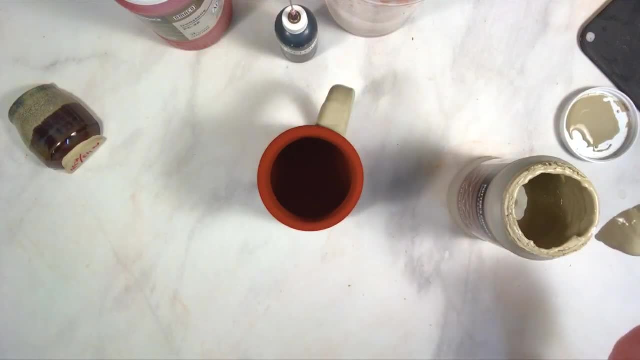 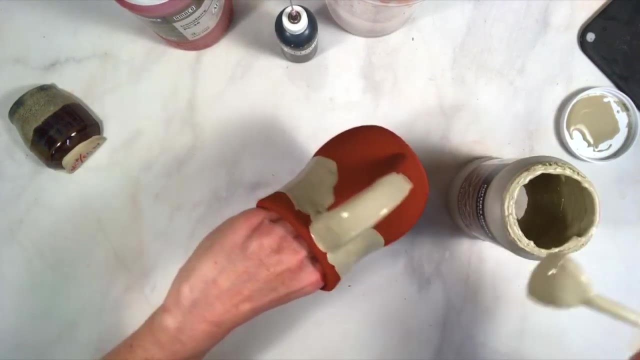 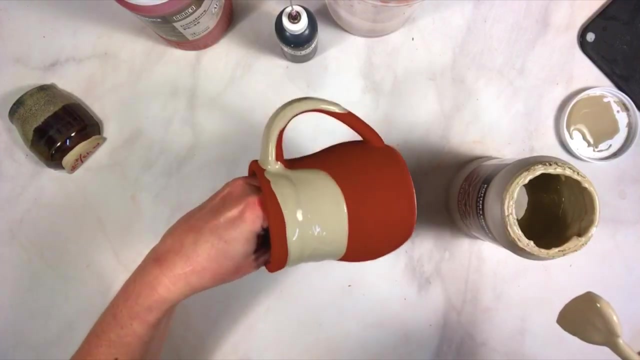 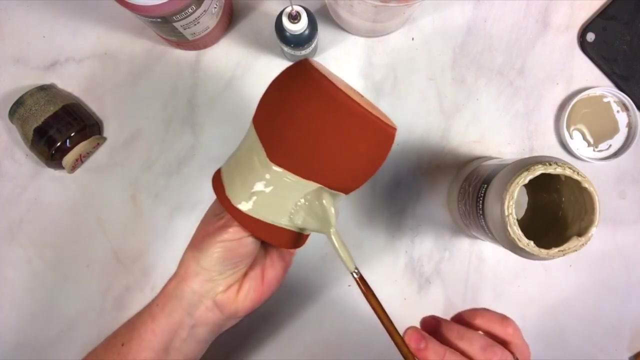 Or where it won't be in contact with food or mouths. It's not. I'm not terribly concerned. There's no lead in any Amaco glazes that are in current production, And the only other thing that the FDA is looking at is cadmium, which I do not believe there's any cadmium. 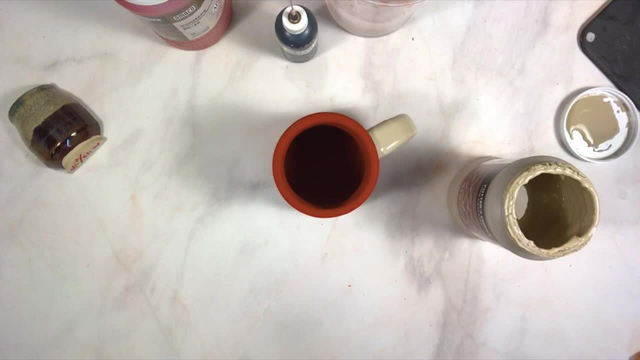 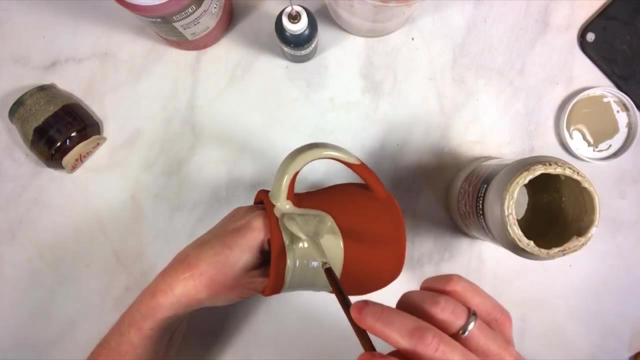 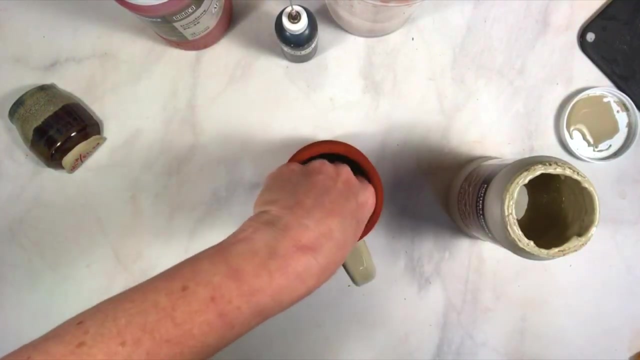 in either of these, And there's no lead in any of these glazes, Pretty sure. So the risk is extremely minimal. But if it's a concern to you, that is the way to do it. So here I'm using the ironstone on the inside. 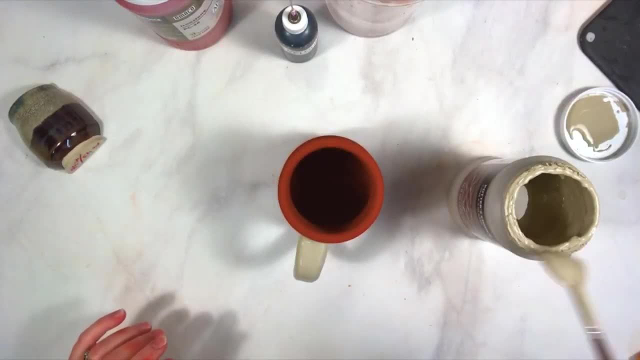 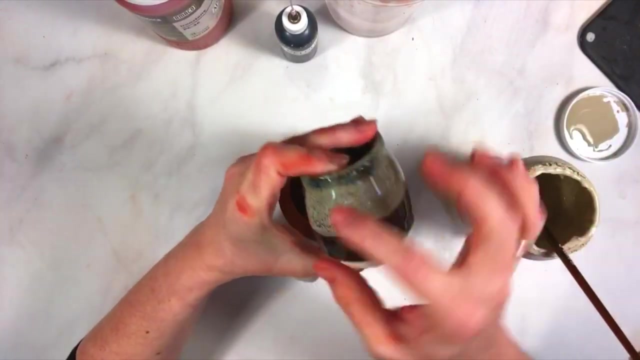 Toasted sage is only on the outside. There's my top coat. I'm going to let it dry a little bit. this can be applied in a lot of different ways, so I could do it on this cup. it was just straight across and you can see it. 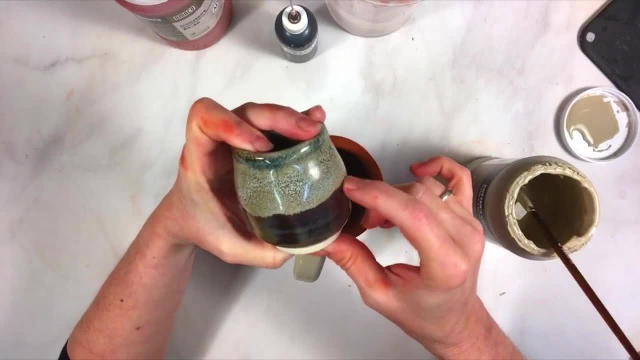 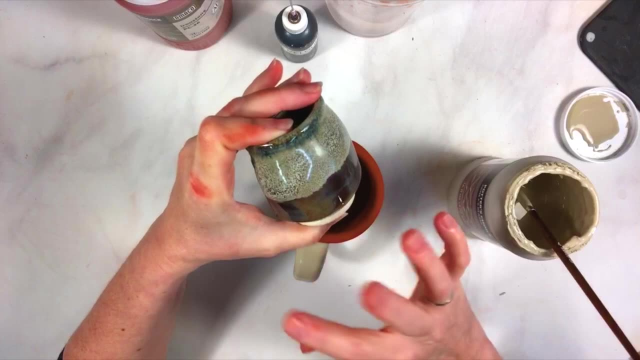 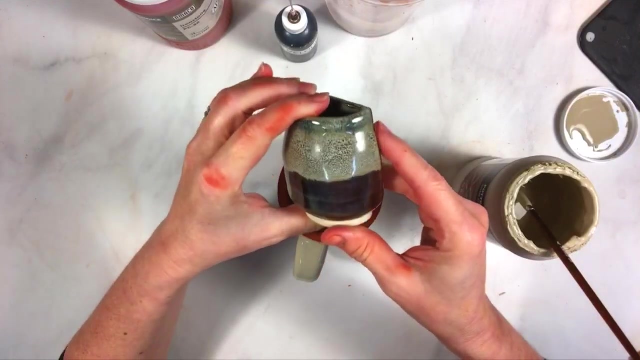 flowed down a little bit on one edge, but it stayed more or less where I wanted it. it could be applied in stripes. it could be applied in dots. if you have a textured surface, you could maybe apply it over the tops, but not into the interstices. so you get a different effect depending on what you were. 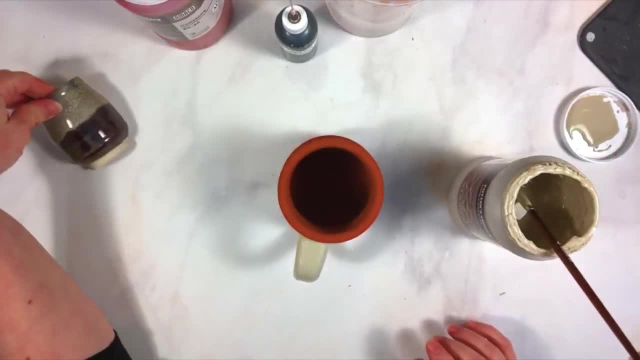 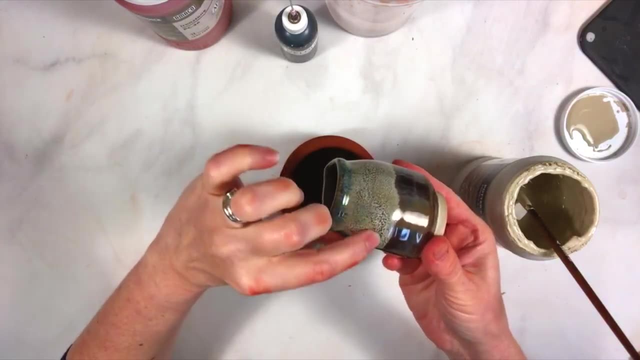 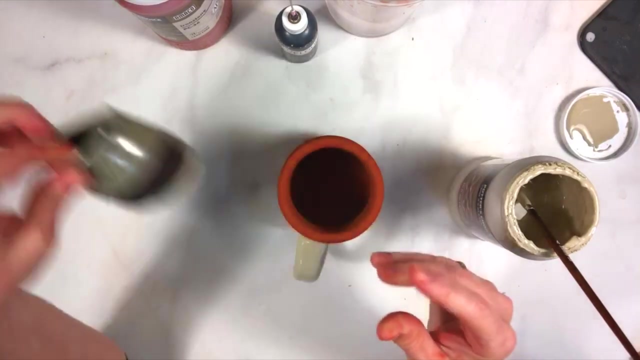 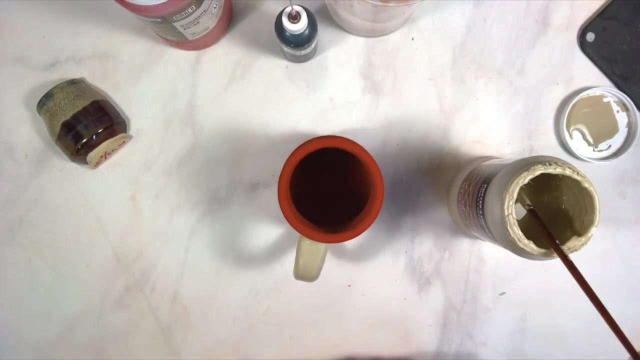 wanting to do. as it's thicker, it'll have a different. it'll have a little bit larger spot happening. where it's thinner it tends to be a little bit smaller. so I didn't have any questions this morning, but I just wanted to say I'm so glad to have people joining me.